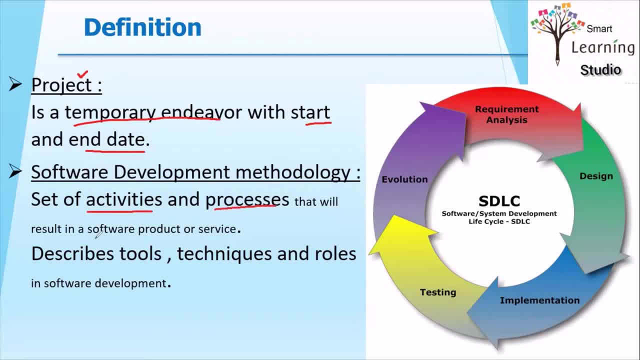 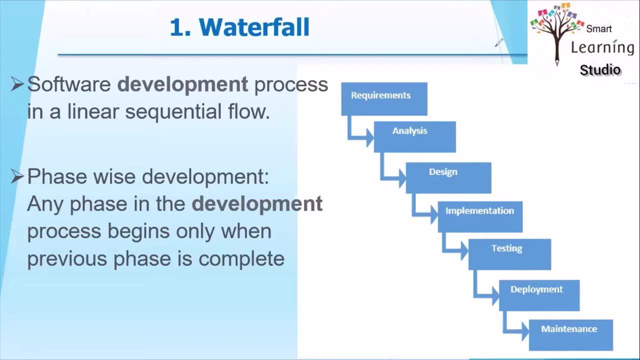 activities and processes that will result in a software product or a service. finally, it rolls around tools, techniques and roles. let us start with the first method, which is waterfall method. as the name indicates- waterfall- you can see that all types are here in a ladder form. so all processes are in a ladder form and it's like a free flow of water. 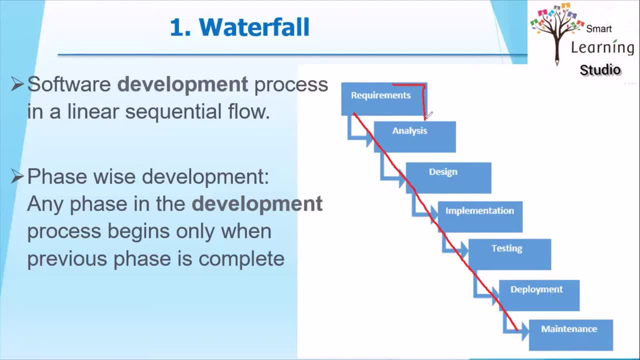 you will see that when one of the process is completed, second one of the processes is completed, that is a valid process and then a withdrawal process will start. so like this, it will come. so that's why it is called as waterfall method. so this processes in a linear, sequential flow. it has a phase wise. 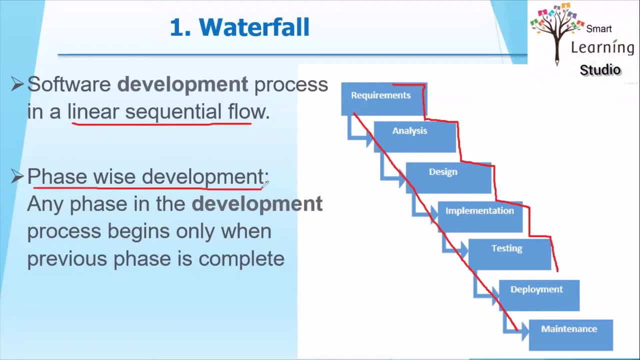 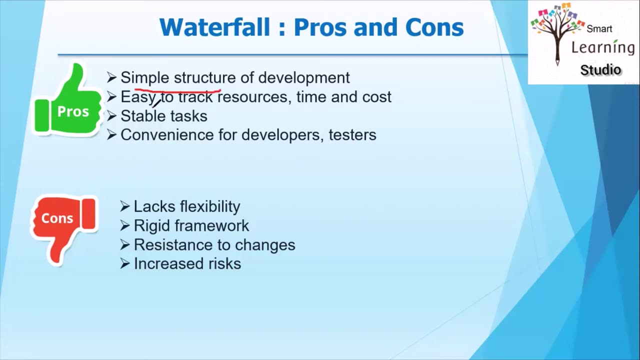 development. this means that when any one of the phase will complete, then only the next phase will start. it is one of the very old methods. pros and cons of waterfall method. it is very simple as you can see, very easy to track resources, time and cost. it gives stable tasks. it is very much convenient for developers. 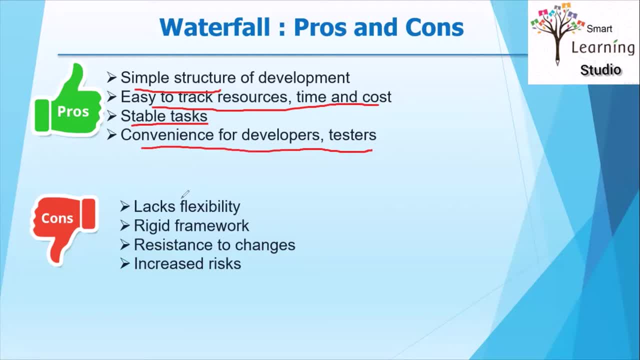 and testers. what are the cons? less flexibility. it has a rigid framework, a resistance to changes and increased risks. so we can see that this is a very simple method, generally useful for very larger projects, but it is very rigid. changes are not easy in this project. let us come to the next one, which is agile development as the name. 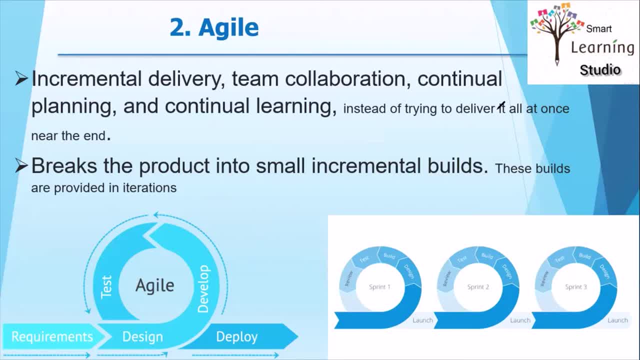 indicates? it indicates incremental development and delivery. you can see that. let us start with the picture first. requirements are gathered, design is done, development is done, testing is completed and it is deployed. so short phases, cycles are completed and this iteration continues for the complete project. so we can see that it has incremental delivery. team collaboration is good. 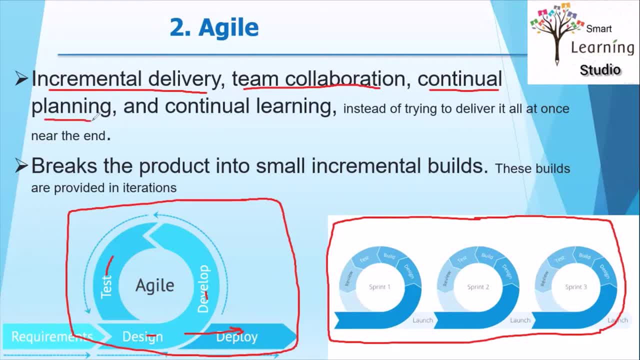 it is continual planning. since you are developing very small and submitting and there is a continual learning process, it overall breaks the product into very smaller incremental builds. these builds are provided in iterations, so in a way we can say that small, small development, testing and deployment keeps the project going on. let us 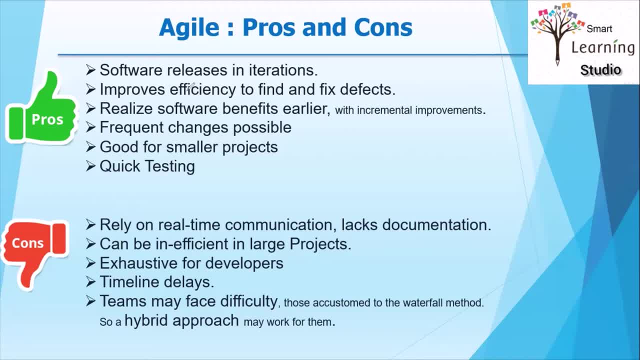 discuss the pros and cons of agile development. software releases are in iterations, so this is a good thing. it improves efficiency to find and fix defects, realizes software benefits earlier with incremental improvements. so you are developing very small, small parts and testing it and deploying it. so risk is less, it is giving better results and it is improving the efficiencies. 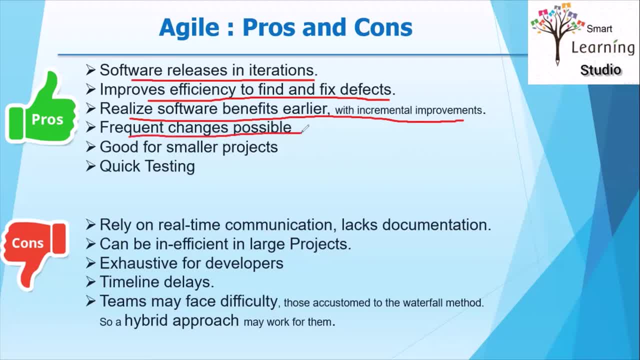 frequent changes are possible so you can incorporate the changes while you are developing. it is good for smaller projects. quick testing is possible. now let us come to the cons of it. it relies on real-time communication, lacks documentation, so you can understand when the time is very less and every day you are developing, testing and deploying most of the time. 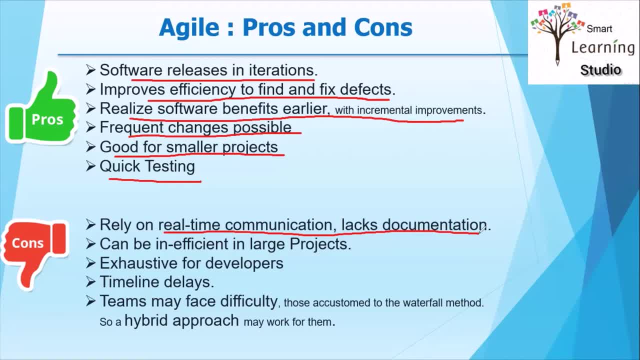 you are in the discussion mode and documentation goes for a bad seat. it can be inefficient for larger projects, so you can understand when projects are very large you can't deploy small, small things. you have to have big chunks of development, testing and then deployment. so this type of development is 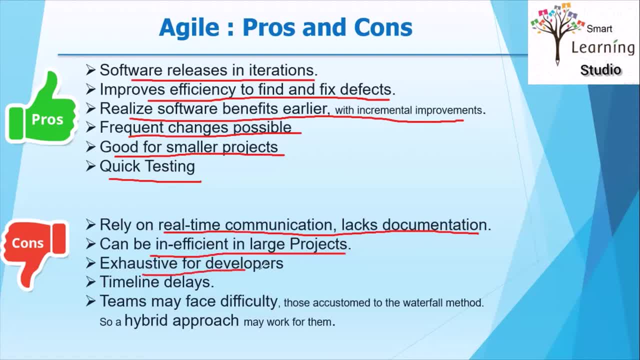 inefficient for larger projects. it can be exhausting for developers. so you can understand that every day, every day, they are developing, the testing is going on, deployment is going on. again next day development starts. so they don't have time. there can be a timeline delays because new developers are emerging. you can see the data. it can be used in different ways to complete your 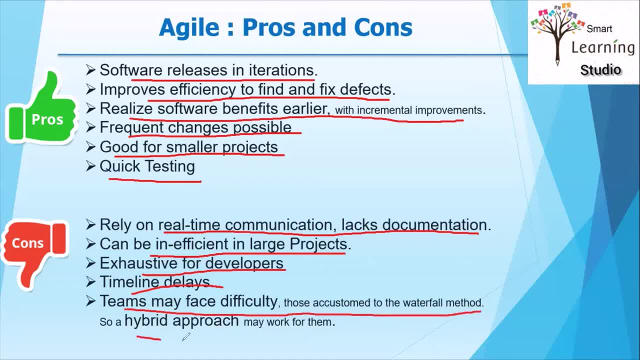 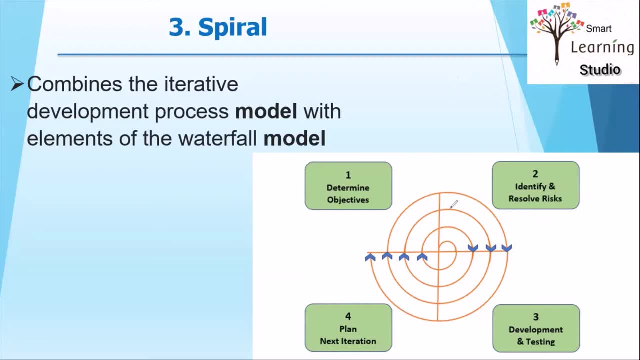 project. for example, there is a specific project which is already in development which you can have time for the next day, and then you can go and test the device through a lab. so this way it is not difficult. you can. Lily, can you please go to the next slide? 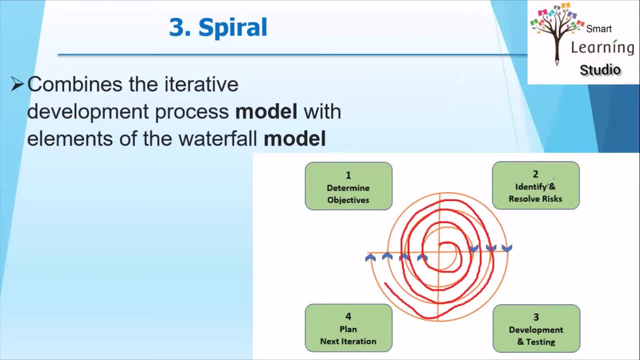 so in this case this is the TensorFlow state- the kind of study of this project has been launched: identify and resolve the risks, develop and test and then plan next iteration. so the continuous stages can be there and you can be like in two, three phases of continuous development. let us discuss the pros and cons of spiral method. 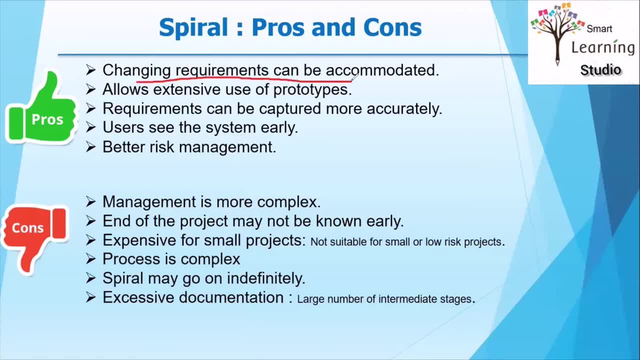 changing requirements can be accommodated. so this type of method can be good where a lot of requirement changes are coming up, so you can accommodate and develop into the next iteration. it allows extensive use of prototypes. requirements can be captured more accurately since you have time for it, users see the system early. it has better risk management. now coming to the 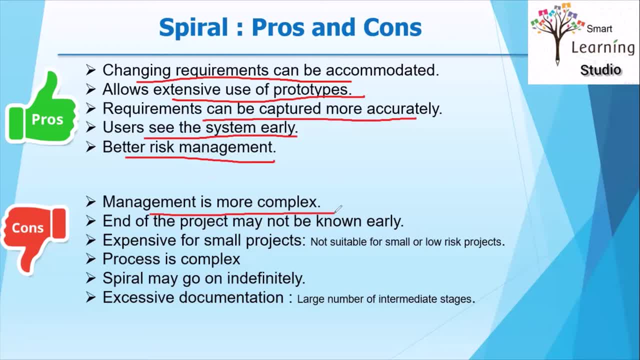 cons of site management is more complex, since you are in continuous development. you are working in a spiral mode. different phases are working at different times, so complexity will increase. end of project may not be known earlier. so this is very important thing, because you are in iteration development and you are 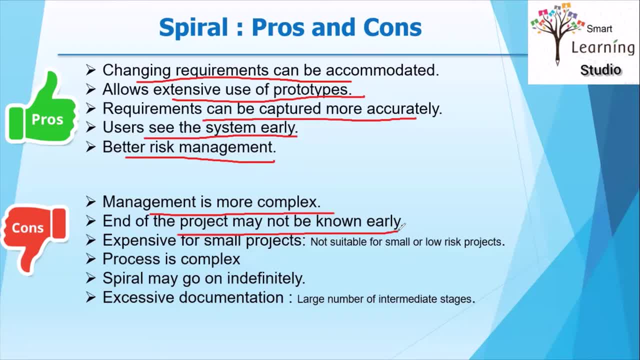 working in a constant spiral development. your project delays may happen. it is expensive for smaller projects, not suitable for smaller, low-risk projects. process is complex. spiral may go on indefinitely, especially for in-house organizations. if the development starts and you are in constant interaction with the customer directly, new changes may keep on coming and then it requires an excessive 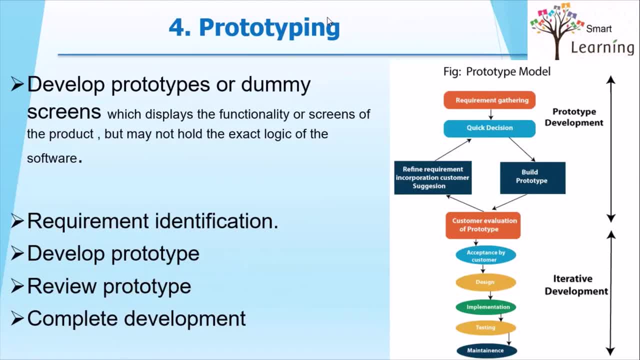 documentation. our last discussion method is prototyping. in this prototyping, as the name suggests, you develop prototypes or dummy screens, which displays the functionality, all screens of the product, but may not hold the process for long time, exact logic of the software. so this is a very common practice nowadays also, and 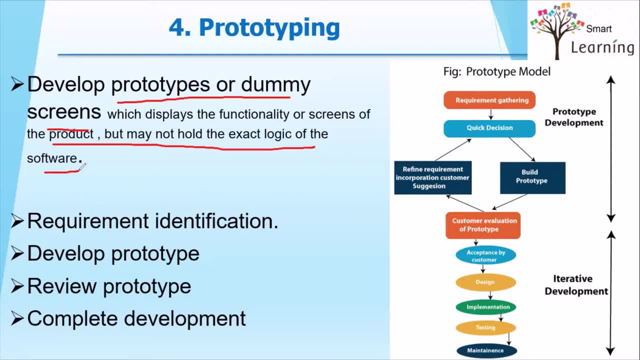 for customer also. it is very easy what happens whenever there is a requirement. sometimes there might be understanding gap with the customer. so in this type of prototyping method you just develop a prototype screen, display it to a customer and he can immediately approve or suggest changes on this. so you can. 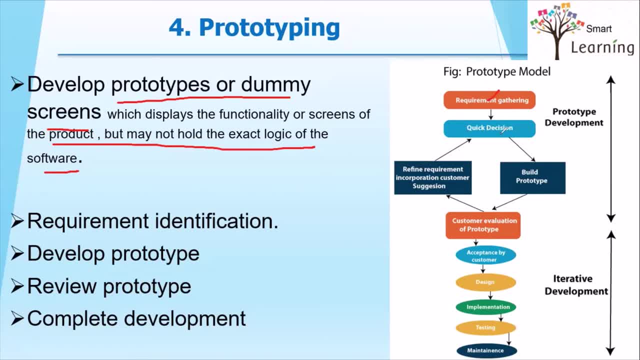 see your the diagram. also, there is a requirement gathering face quick decisions there. you build a prototype, you get it evaluated. if it is not correct or require some changes, you again go and make the changes. so this cycle continues. after that, customer evolution of prototype is completed, acceptance is taken by the customer, then design and other phases are there and 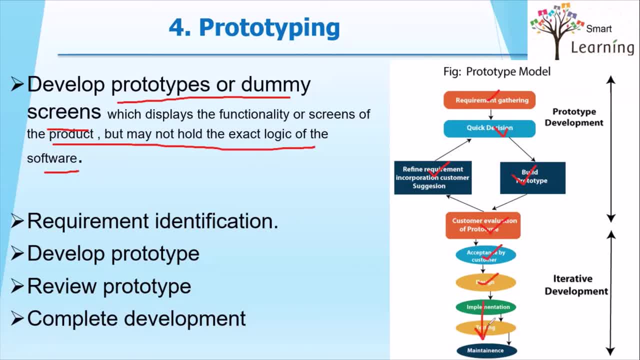 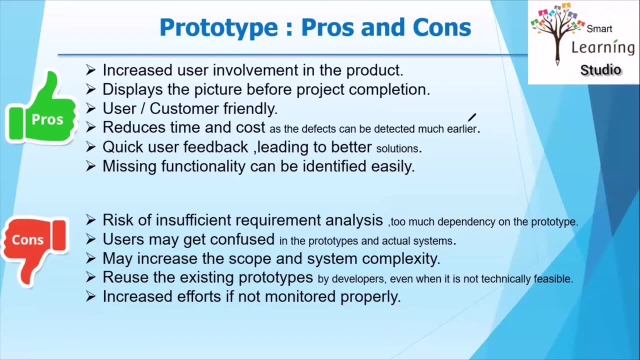 you declare the project so one of the good ways which is now being entertained. it has different phases, so requirement identification, develop prototype, review prototype and then complete the development. let us discuss the pros and cons of prototype method. in this there is increased user involvement in the product. it displays the picture before. 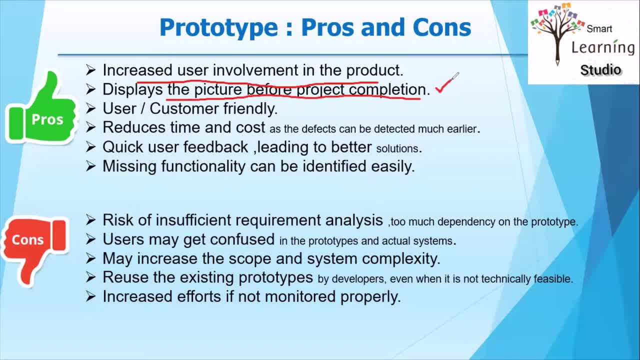 project completion. so very much helpful for customer since he can see the prototype screens, he can understand what is being developed, rather than when the project is completed and then you see the result. so in this way it is very much user and customer friendly. it reduces time and cost as the defects can be detected much earlier. you get a quick user feedback leading 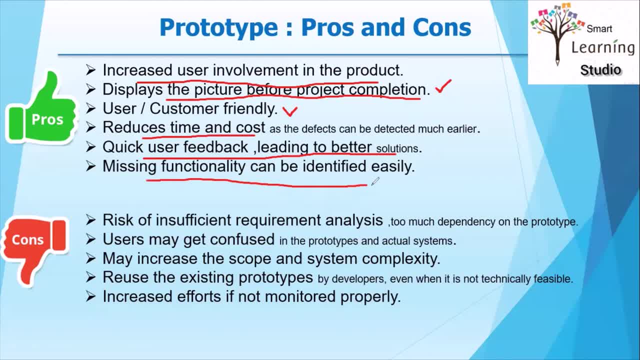 to better solutions. missing functionality can be easily identified. so in this way, a lot of benefits you can see out of this prototype method. now coming to the cons: risk of insufficient requirement analysis, too much dependency on prototype. so in this, what happens when you know that your customer is there and you can show him the picture? 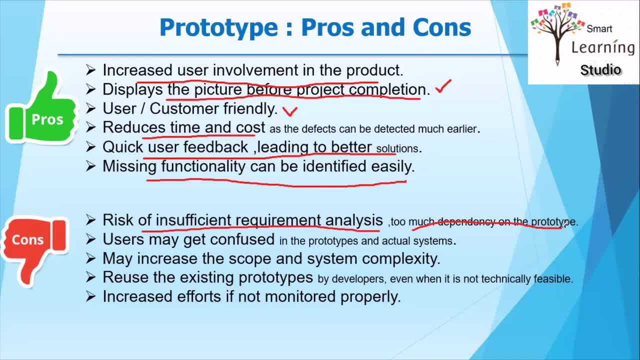 so you don't go into lot of requirement analysis and gathering. this can be a negative thing. users may get confused in the prototypes and actual systems may increase the scope and system functionality or complexity. also, there is a tendency in developers to reuse the existing prototypes. this can be dangerous or sometimes not technically feasible.